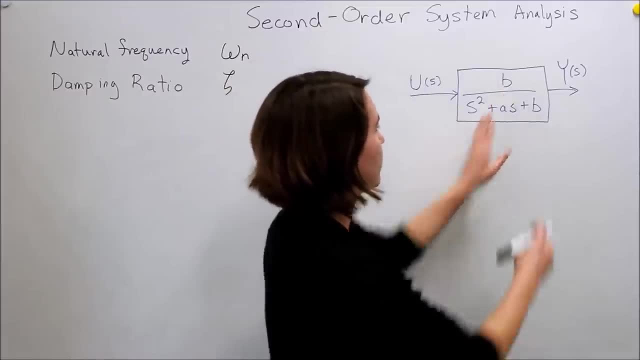 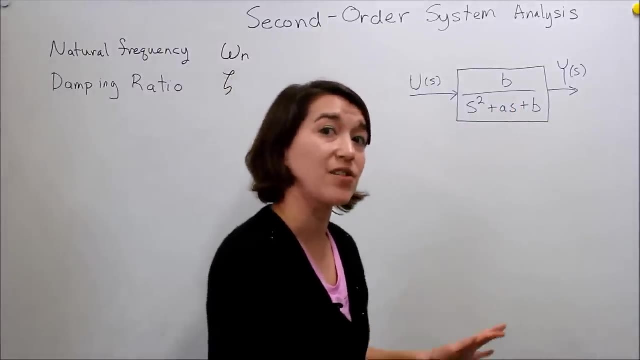 is the denominator. We know that if we have s squared and only a, b, so if a is 0, then we will get some oscillation because we'll be on the imaginary axis. Our poles will be on the imaginary axis. So b roughly correlates to omega here. 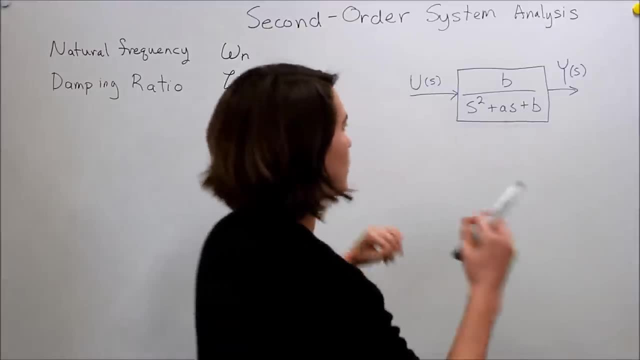 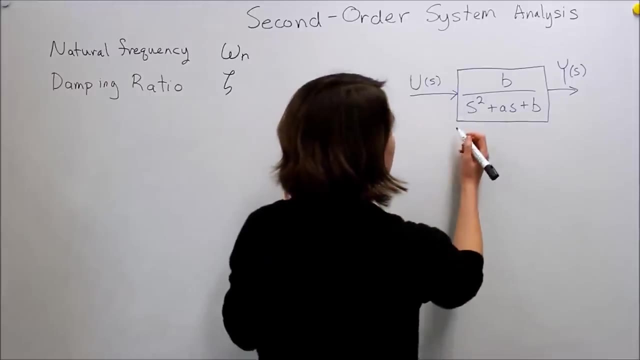 And then the damping constant comes into play with this a, So I'm not going to drive the whole thing. If you want to see the derivation, you can do it yourself or look in a book, But what we end up doing is rewriting this system. 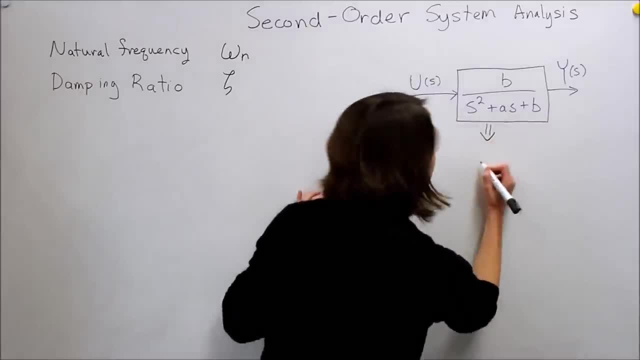 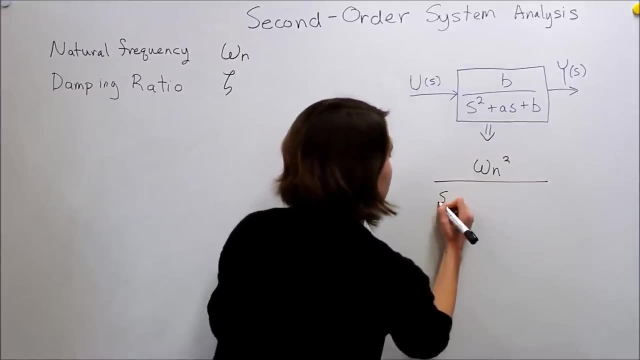 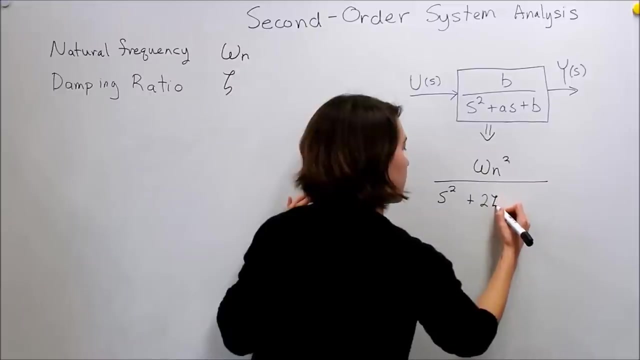 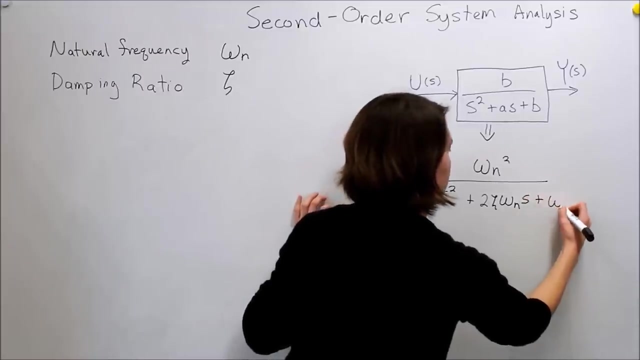 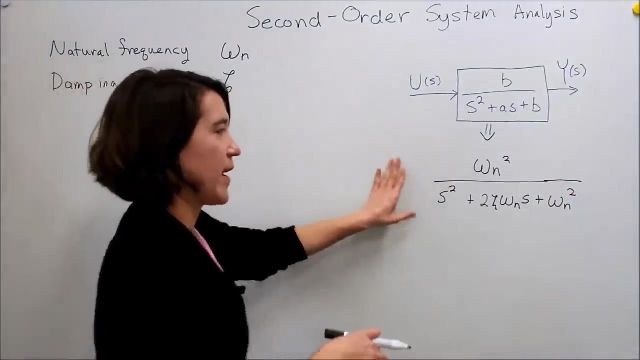 So this ends up looking like omega n squared, so the natural frequency squared in the numerator, And then we have s squared here And then a will become 2, the damping constant, omega n s plus omega n squared. And we're going to do a little bit more analysis. 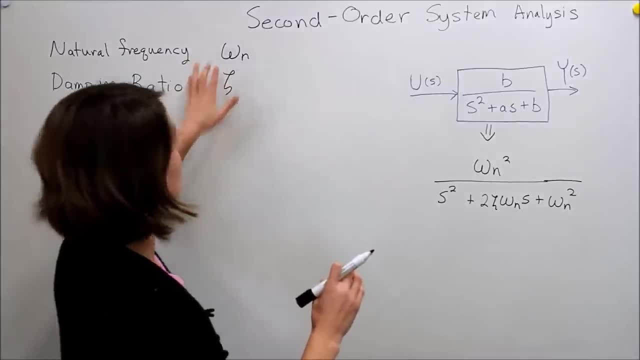 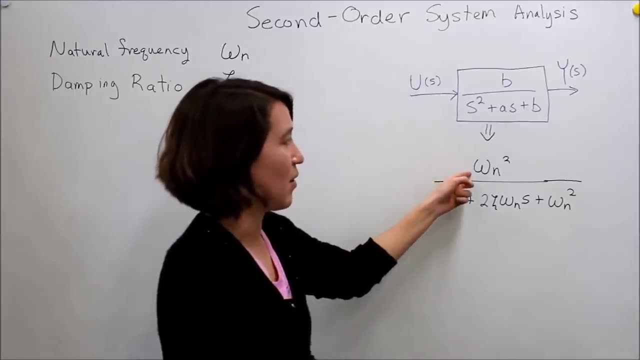 But essentially what we do is we understand these things or we will. We'll talk about them more And we've got to force them into this equation And we notice that it's like this omega n and this omega n are the same. 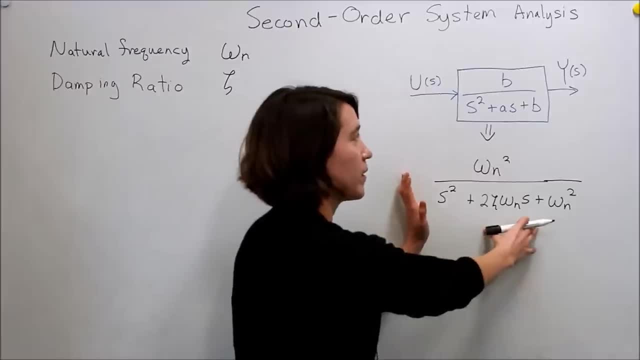 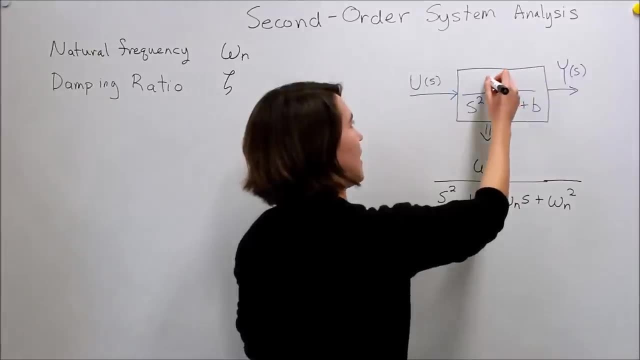 And you can try to fit your equation into this form. But what if you know you might have the question: what if I have another constant out here or something? So we have a constant alpha, or you know, alpha, like this, number does not match this. 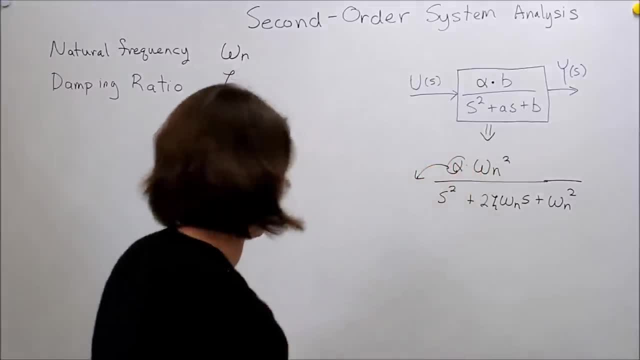 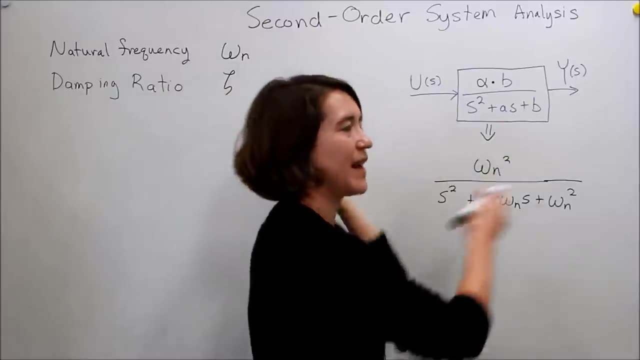 All you have to do is take this and move it to the front so it can become a scalar. So that's just to address that question. So if you want to force it into this form but your top number doesn't match this, you can take out a constant. 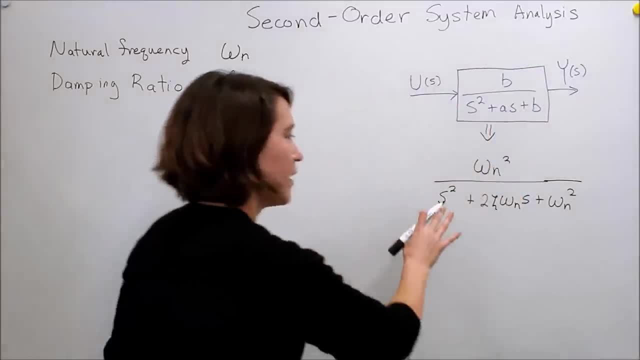 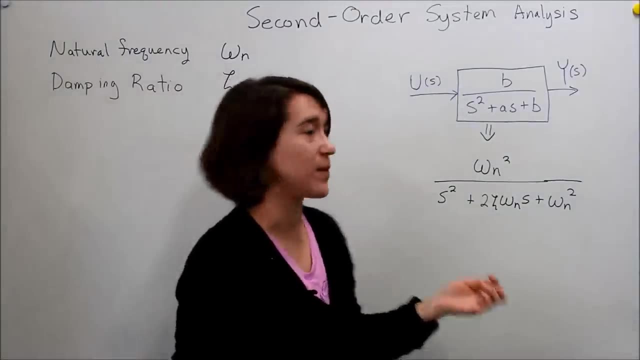 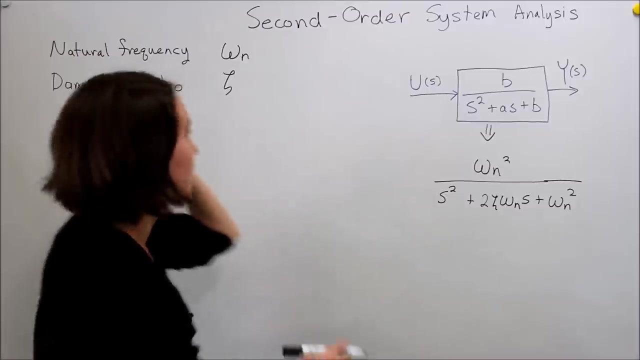 Okay, All right. so say, you can get your system into this form. Well, what do we need to look at? We need to look at the poles, because we care about the stability of the system, So let's derive the poles for this. 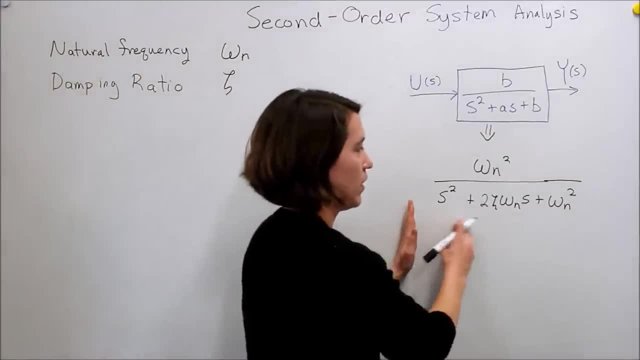 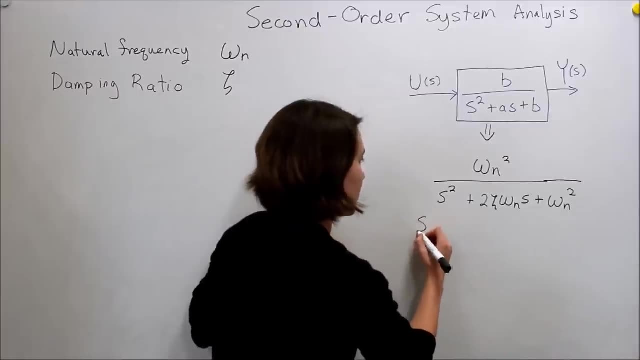 And we will do it right here. So this is general right. So we can use the quadratic equation to find the poles for the system. So we can do s. So this would be a is 1 here, This would be our b and this is our c. 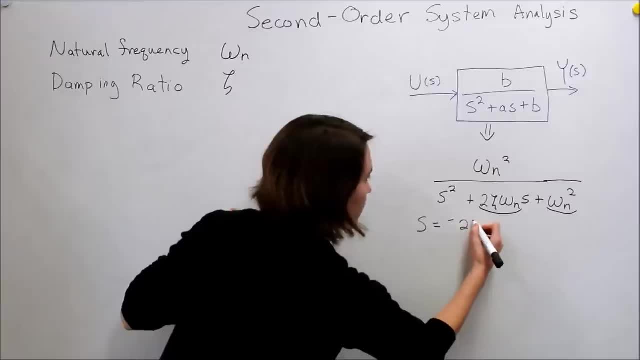 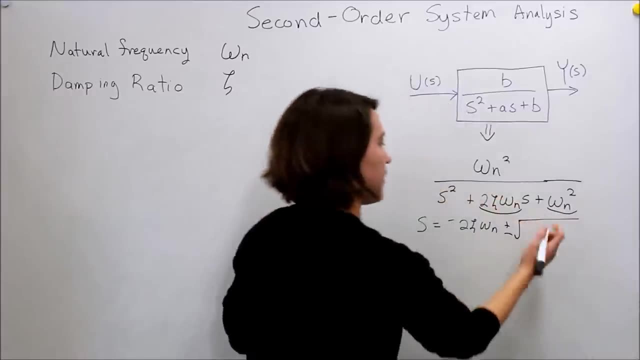 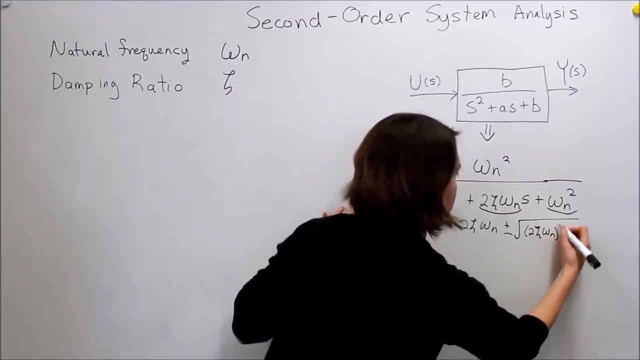 So s equals the opposite of b, So 2, this thing, omega n plus or minus, the square root of This value squared, Oops, Omega n, quantity squared minus 4 times c. so omega n squared all over 2.. 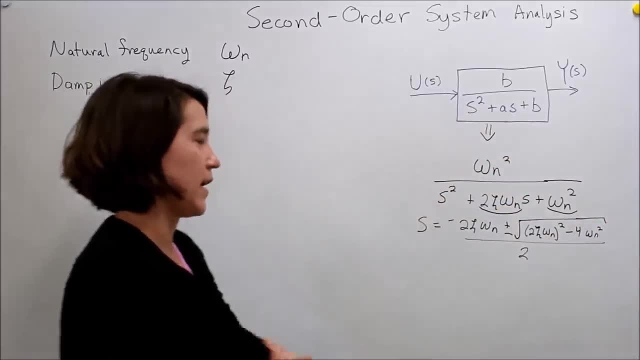 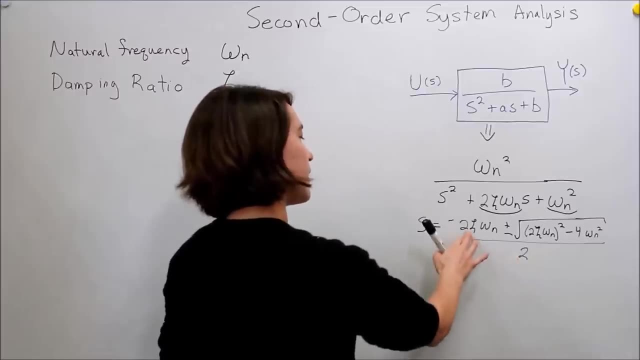 Okay, so we're just taking this. We have it in this form. We're taking the finding the poles. Okay, so if we simplify this, we see that the 2 cancels out here And actually we're going to. 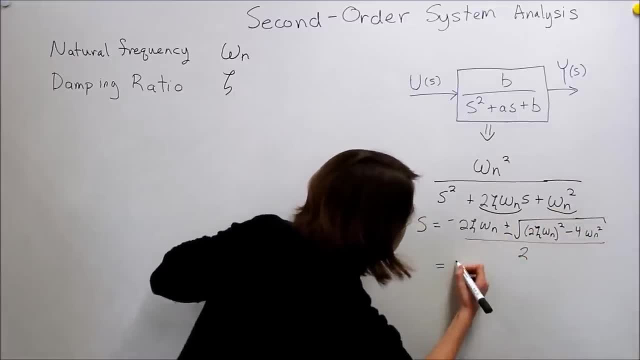 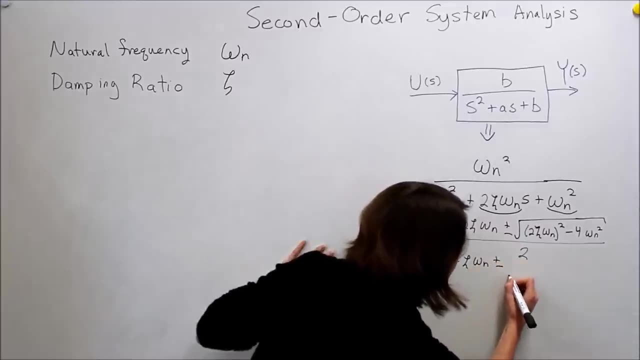 we're going to bring some stuff out of this. So let's first we'll cancel the 2 here, So we'll get negative damping, constant natural frequency plus or minus. this will be all over 2.. And then here we see that there's 2 omega n squared. 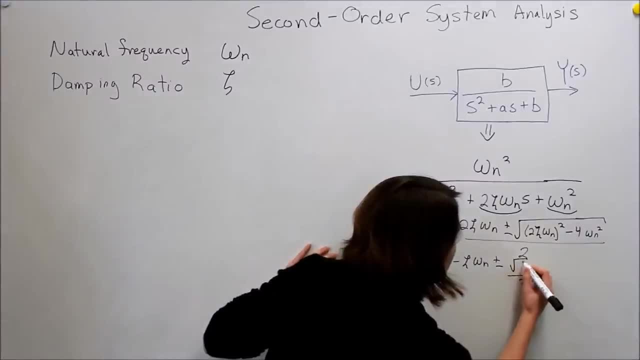 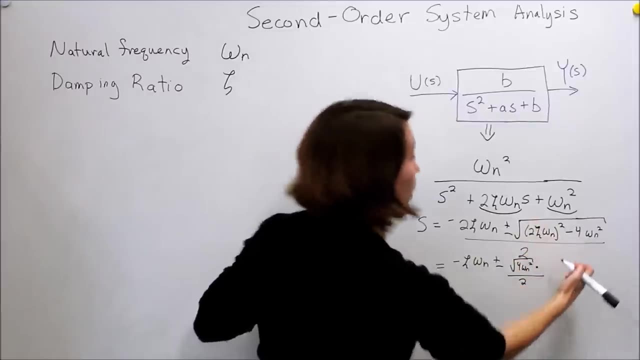 is in common to both, so we can bring that out. So we'll get 4 omega n squared here. times the things that are left here is the damping constant and a 1. So the square root of the damping constant minus 1.. 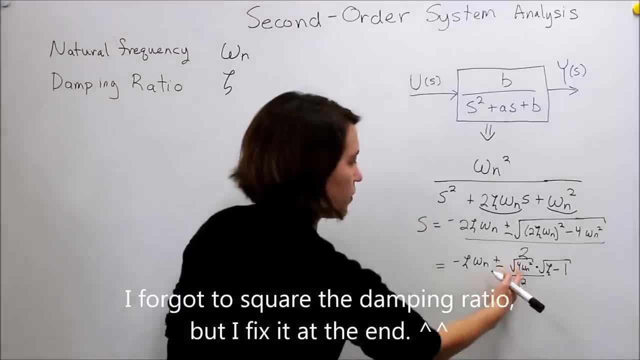 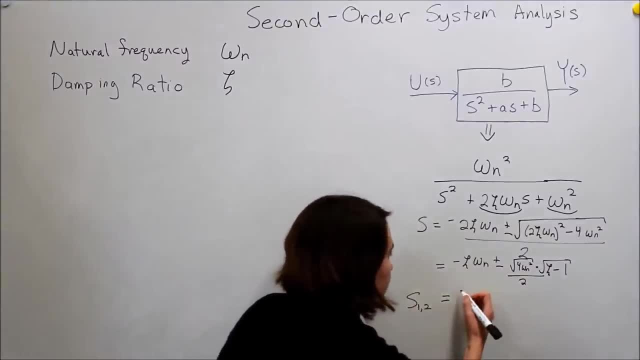 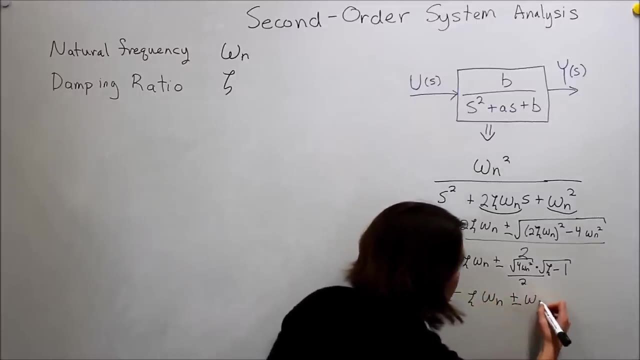 Okay. so if we simplify that further, we'll still get a 2 and an omega n. omega n- the 2s will cancel out, So we'll be left with S12- is equal to negative. the damping constant: omega n plus or minus omega n. 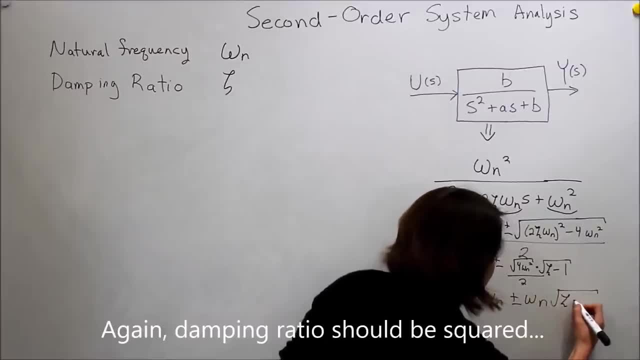 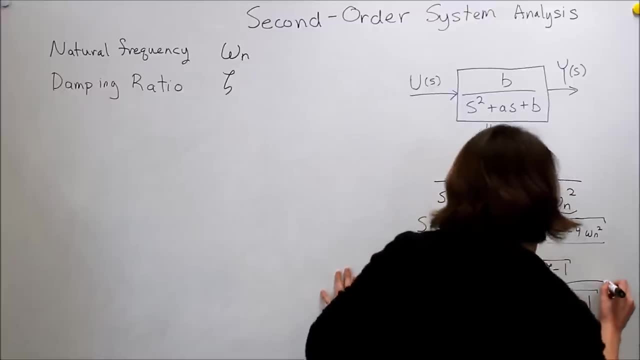 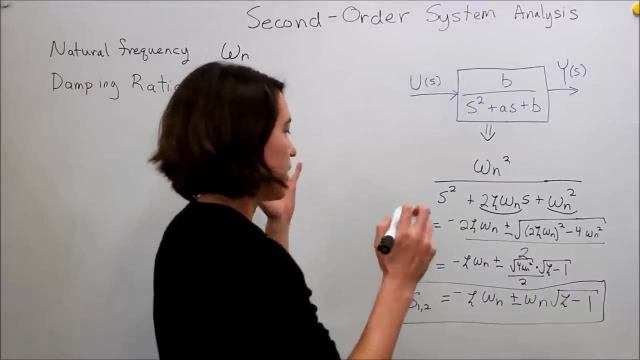 times the damping constant minus 1.. So this is an important equation, because it tells us the poles of our second order system here. Okay, so why did we do this? What's the point of this? Well, one thing that we can see is: 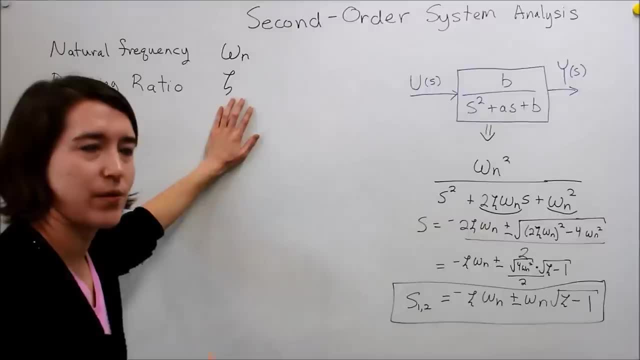 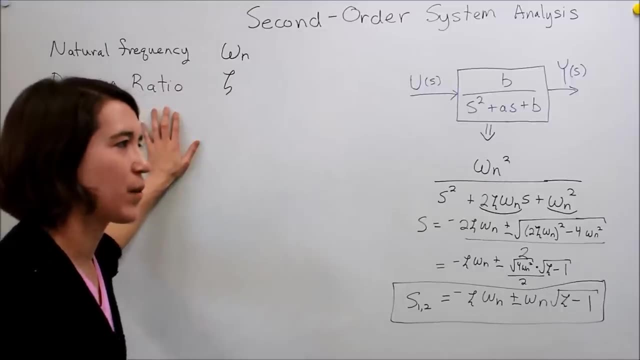 the damping ratio if that's 0, so- and the name kind of gives it a hint- it's about the damping of the system. So if there's no damping in the system, we know that we're going to have an undamped system. 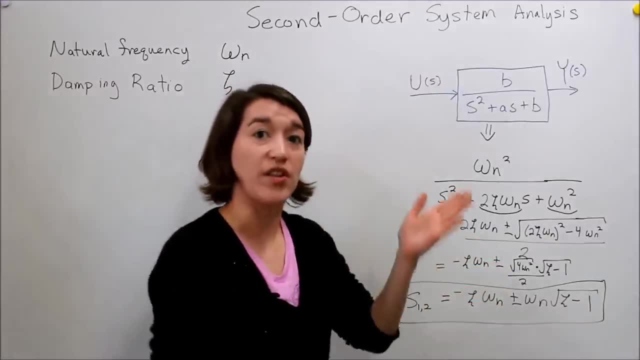 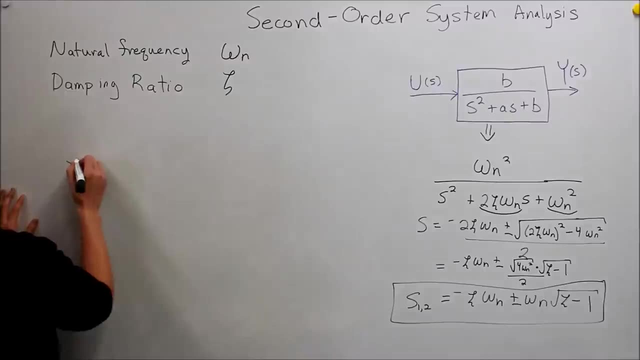 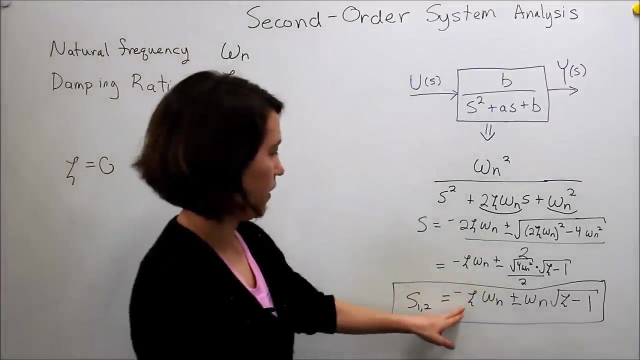 So that means that we're going to have imaginary the poles on the imaginary axis. So if let this value our damping constant, if, for example, it is equal to 0, our poles will be, it'll be negative, 0,. 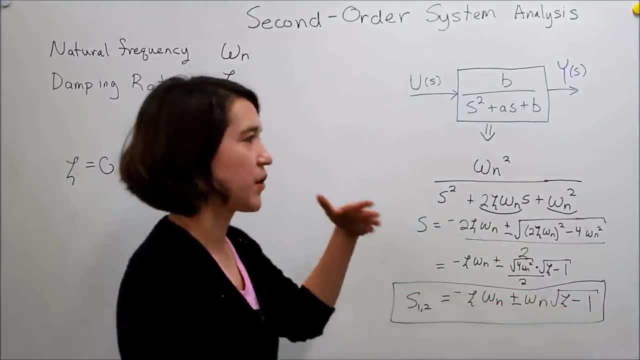 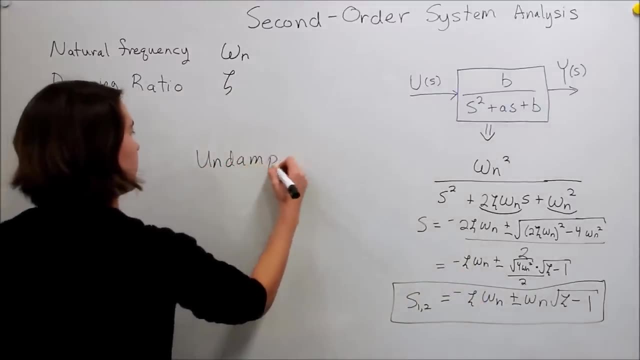 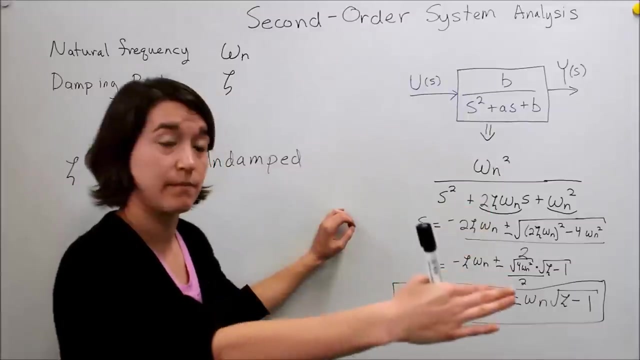 plus or minus an imaginary value here, and so we'll get an undamped system. So kind of makes sense. if there's no, the damping constant is 0, then the system is undamped, it's just going to oscillate. 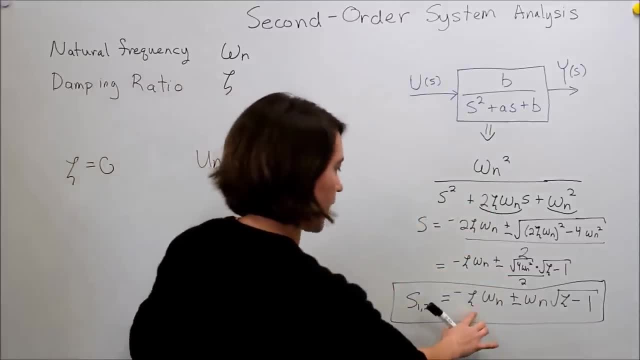 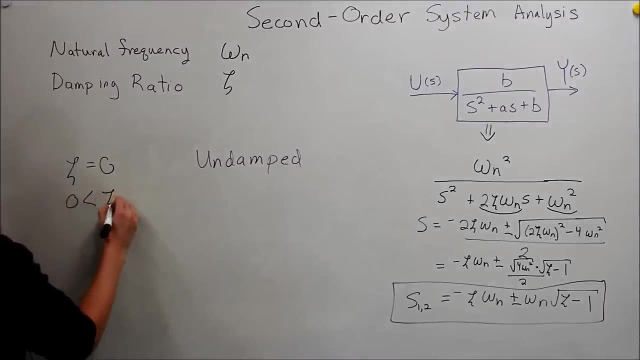 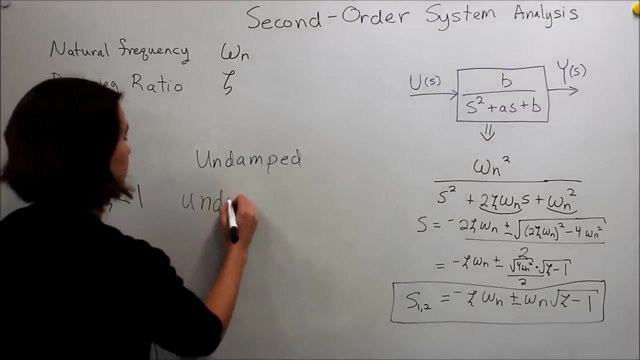 Okay, Well, let's see what else we can do. What happens if our damping constant is in between 0 and 1?? So if we have in between 0 and 1, then we get an underdamped system. And remember that means we have some oscillation. 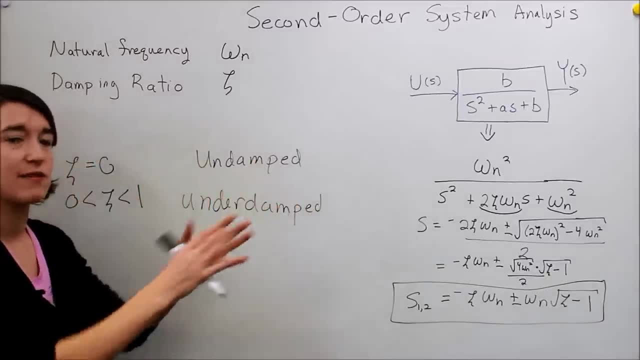 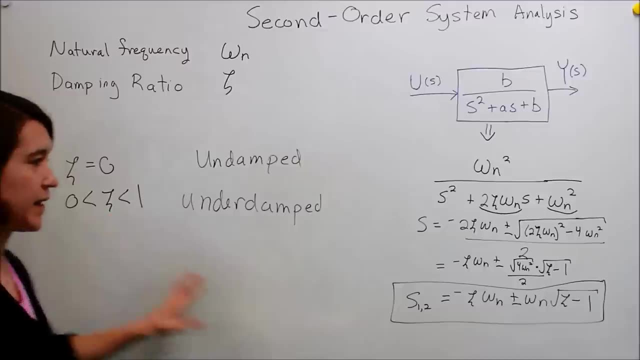 and it eventually gets to our objective point, our target point, but it takes a little bit of more time and it oscillates. So if we look at that here, it means this value would still be negative, right, And so we would still get some oscillation. 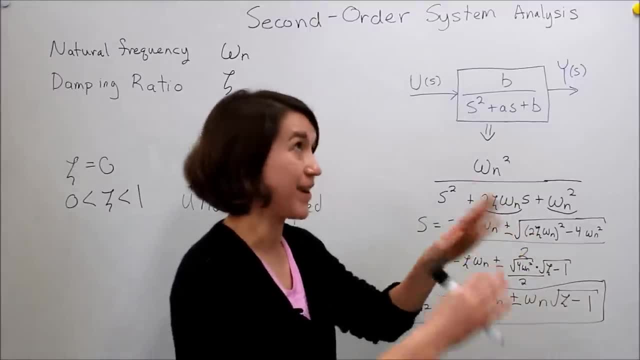 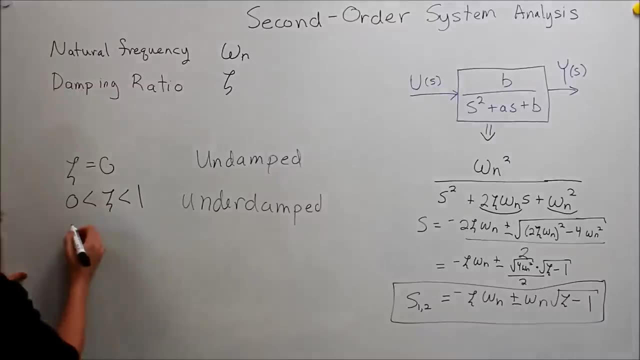 our poles are still in the imaginary axis. sorry, have an imaginary component but are not on the imaginary axis. Okay, Okay. well, let's see what if it's exactly equal to 1?? Well, if we have exactly equal to 1,. 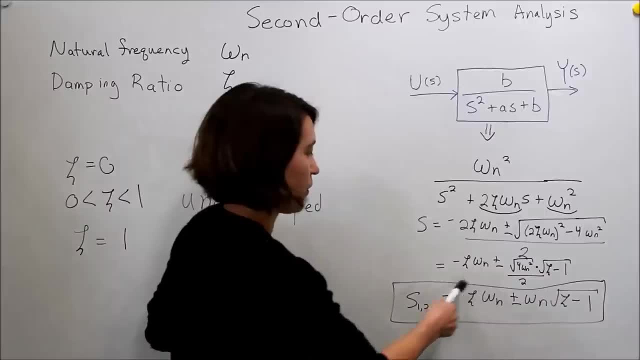 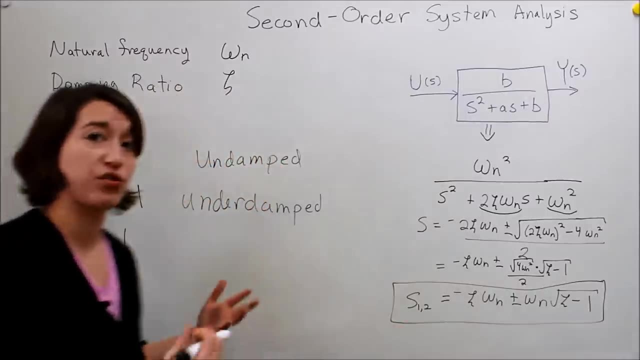 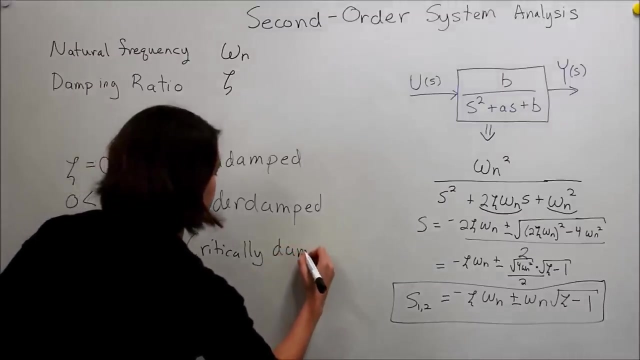 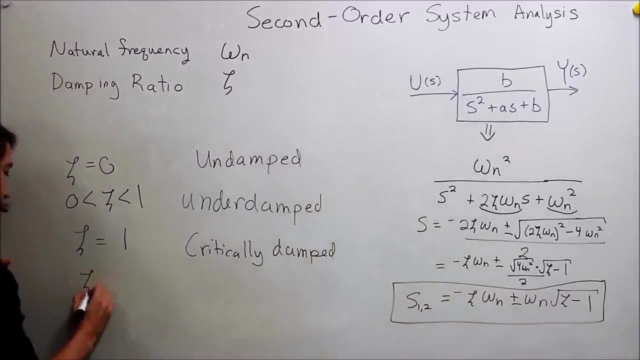 this value would be 0, and then we would just get two real poles on the real axis at omega n. So that would be what we call critically damped. Okay, One more case. what if this value, the damping constant, is greater than 1?? 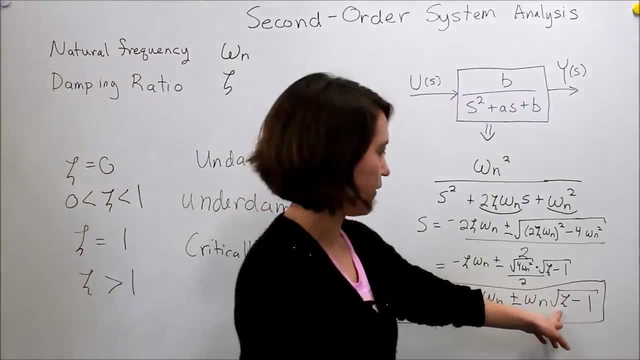 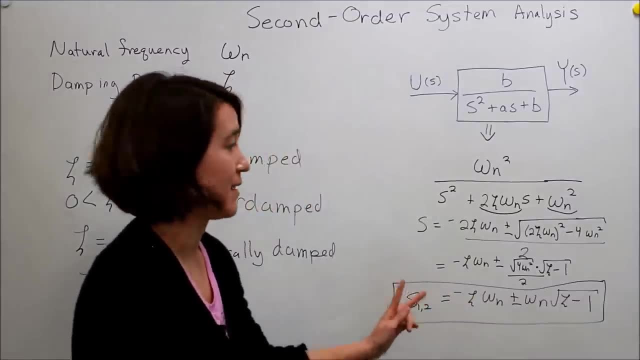 Well, so if it's greater than 1, we're going to have. this is a real value, right? But we'll have two points on the real axis, so it'll be on the real axis, so it'll both be negative. 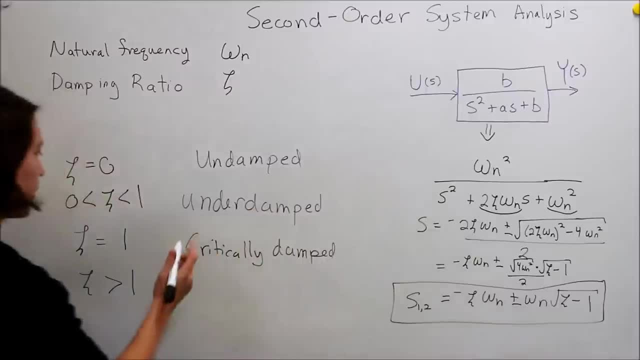 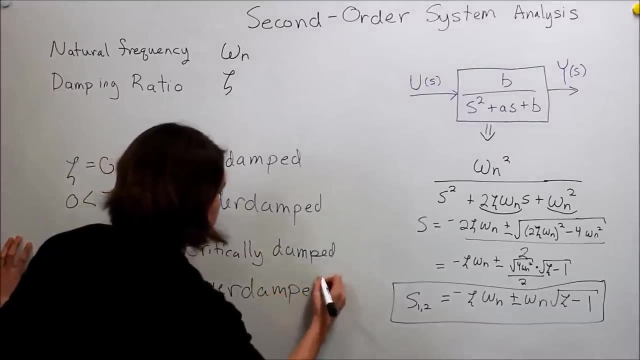 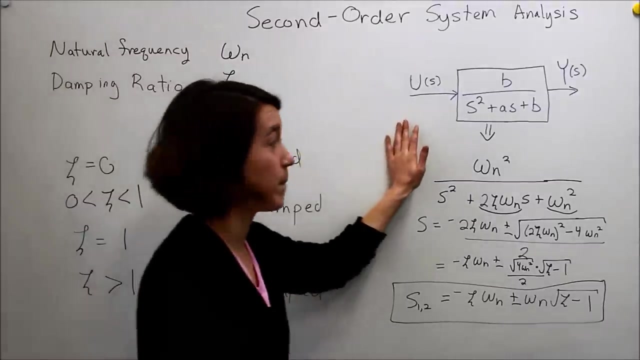 but they won't be the same exact pole, So in that case it would be overdamped. So pretty much what this helps us do is if we have a secondary system that can be put in this form, we can break it down and find these values.